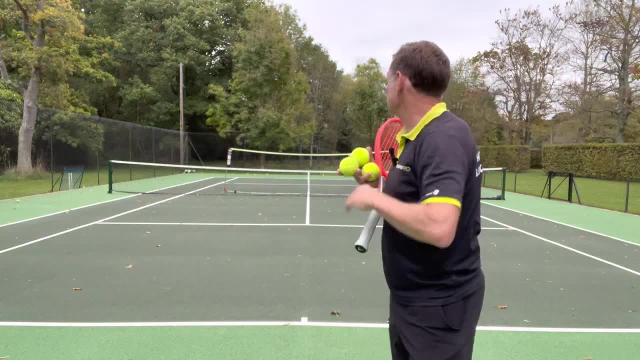 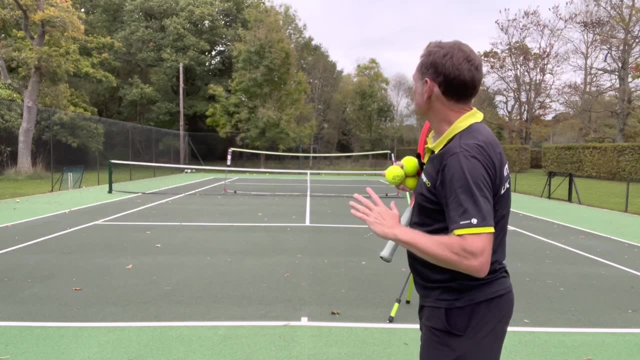 by some distance and I've put a second net above the existing net, almost tried to double the height of the net and now you drop the net forward by 0.25% from your hitting match. Let's try something to the net and just the the, the thought of having to head up like that the nets then making me think. 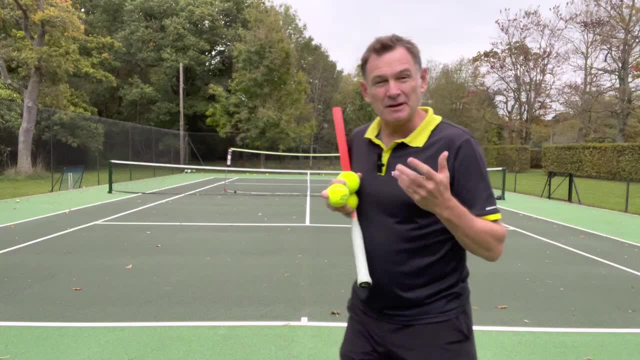 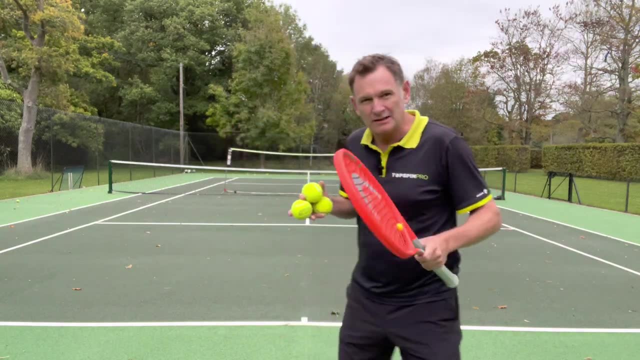 about heading up, uh, and that's what's going to help me hit better tossman technique. now that sounds a bit uh odd. let me explain that a bit better. so sometimes we work on our technique. we we literally focus on exactly what we're doing right here in front of us, how we're moving the 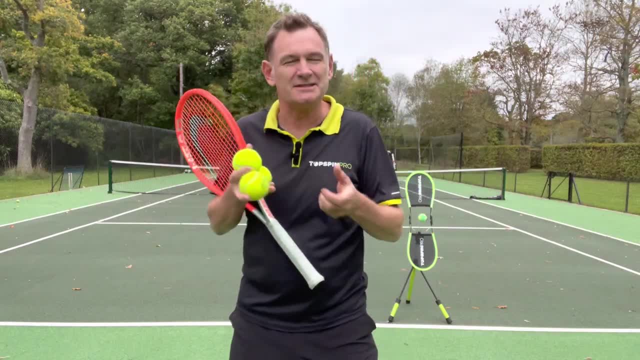 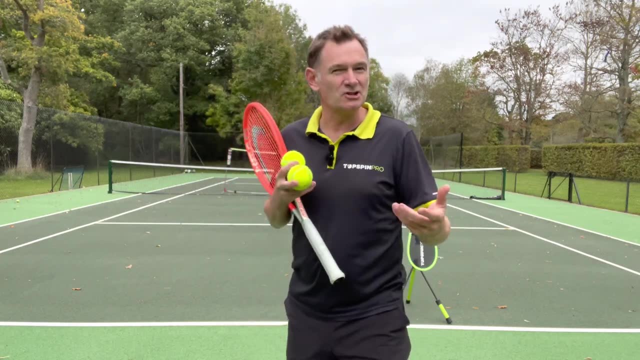 racket we look, we're very much focused on the mechanics and the technique we're using right. it's another way to to work on on your tennis and that's using intention and it's to focus on the outcome. now, often when we learn tennis, we try not to focus on outcome, because if you get too, 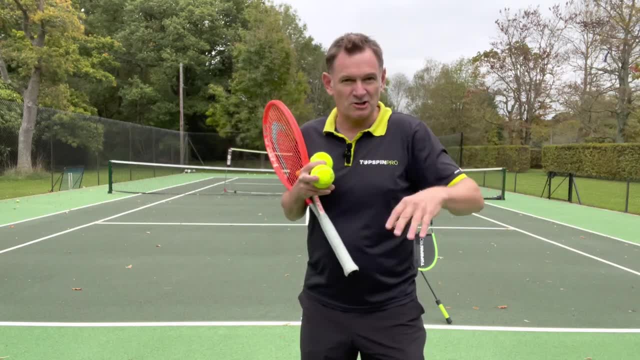 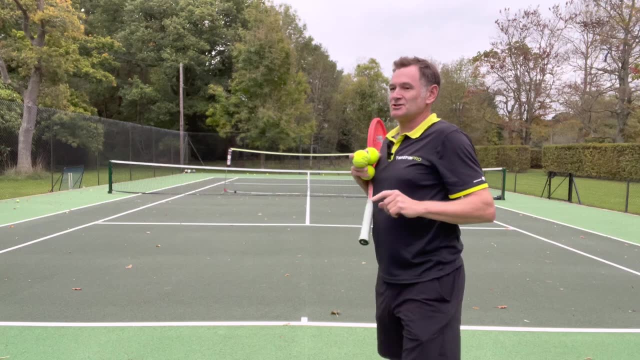 attached to the outcome. you you can't concentrate on the things you're learning, but in this case, the opposite. so we're going to. we've told ourselves we want to get the ball deep, we want to get it into the back box, and by telling ourselves, that's the outcome we're looking for. 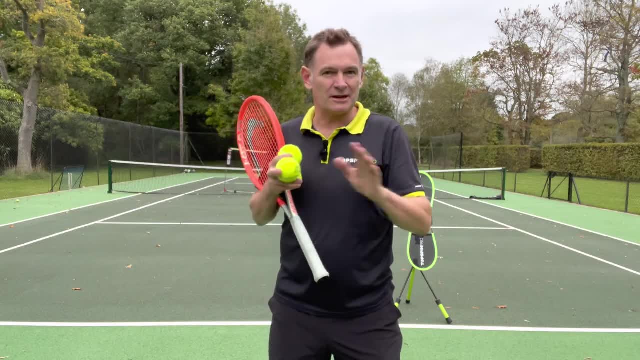 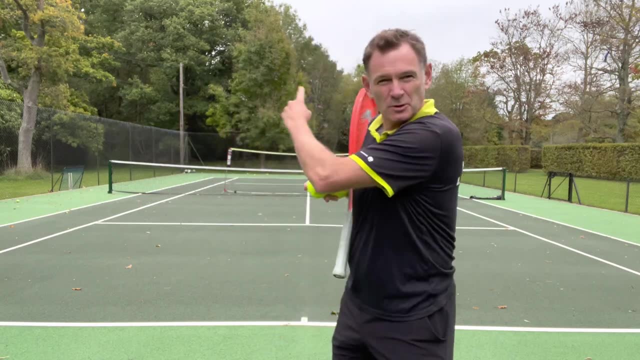 we want to just let the body get on with achieving that. for us it's a bit like the inner game of tennis, that that sort of a logic that's. we want to simplify things, we don't want to think about it too much, we know that's where we want the. 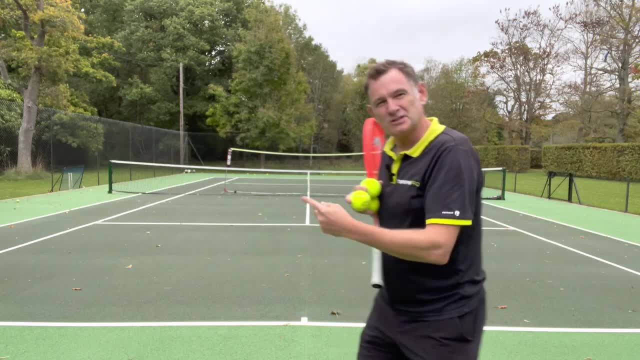 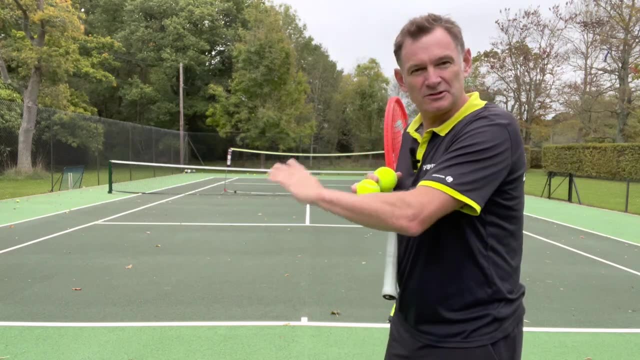 ball to end up really deep with a lot of Topspin. we use the Topspin Pro just to reinforce the sort of right swinging mechanics, just to give us a bit of a guide, and we use it just before we hit the shot. so let me give an example we're going to do. we're going to do 20 of these right. so 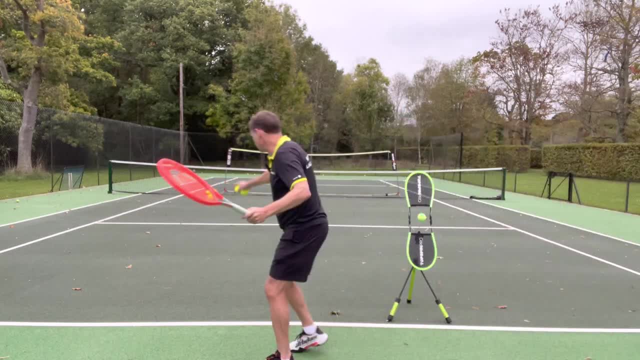 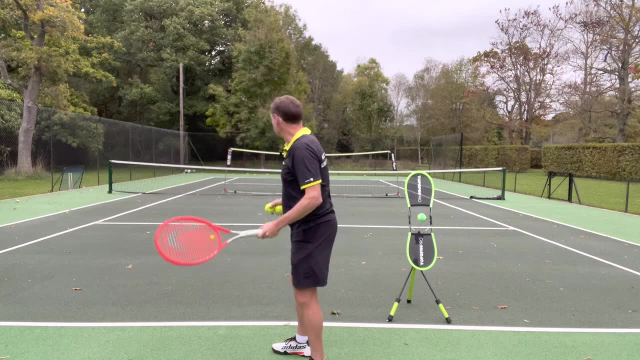 you hit your Topspin forehand like that. then you run across to the side, drop the ball and hit it. okay, that's really deep. probably a bit too much, uh, height there, but the idea is to use that net to make you think about hitting up right. the Topspin Pro also makes you think about hitting. 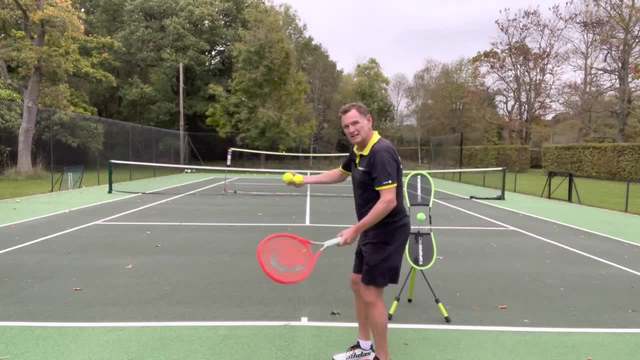 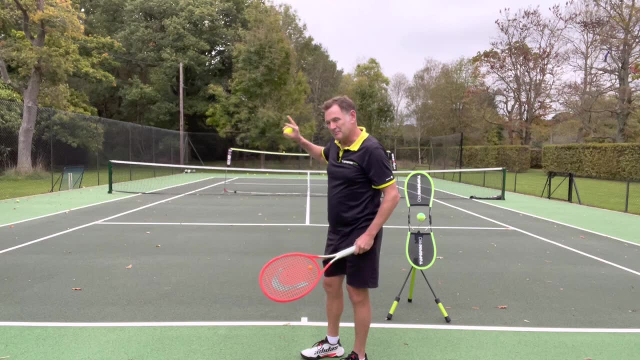 up. so a couple of goes on. the Topspin Pro jump to the side while that muscle memory is fresh. straight away, it's that shot. you've got to clear both nets and by doing that you're much more likely to get the ball into the back box. there we go. 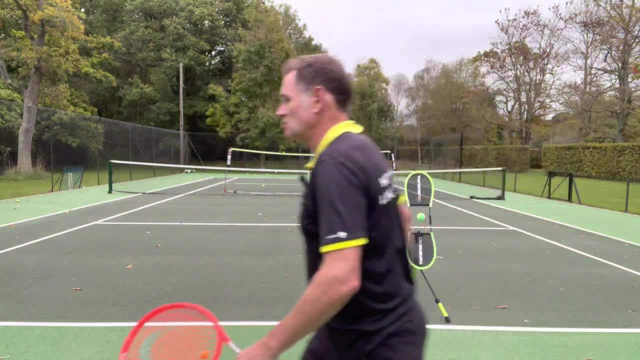 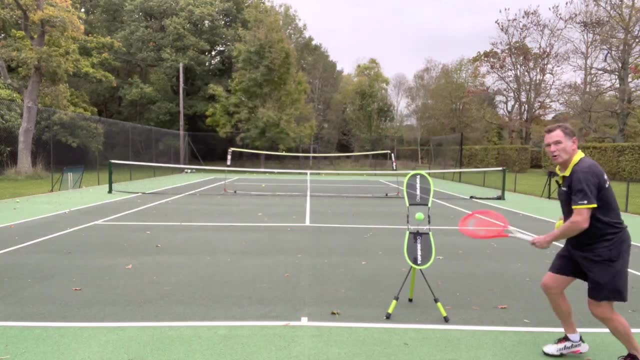 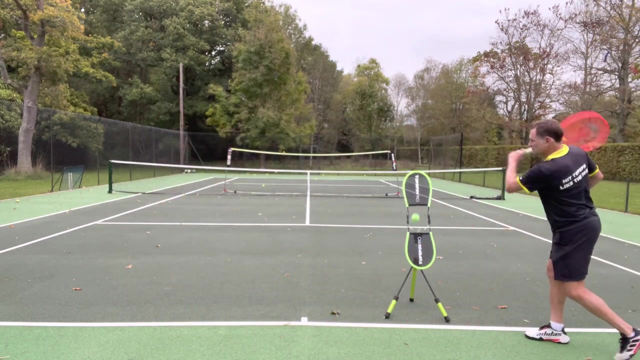 so it's a great drill to work on that and you can sort of mix it up a little bit, right, so you grab a few balls there. you can play your first shot in the Topspin Pro. run across here, drop the ball in front of you, hit that depth. now you can try an inside out forehand so you'll hit the shot. 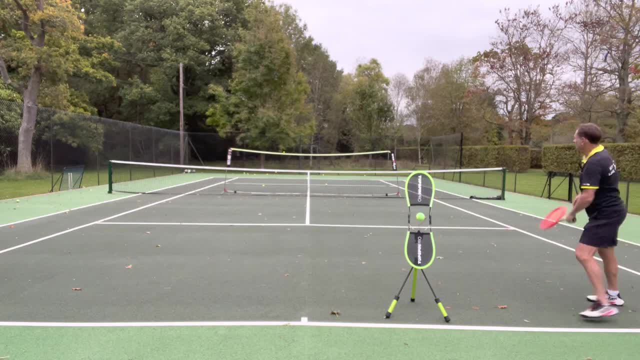 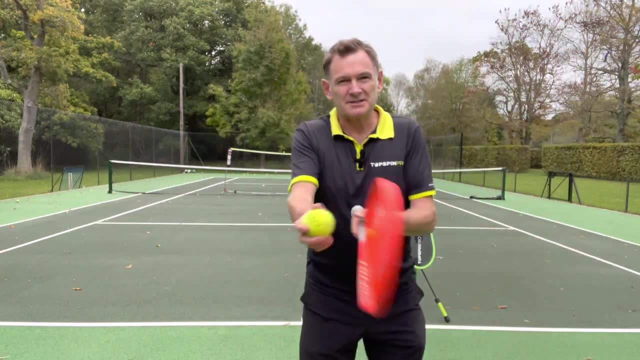 on Topspin Pro. you'll back away like this and do that right, but that visual element of having a net in front of you forces you to think about hitting up. and instead of hitting up like this, you're going to close your string slightly close and that's going to get that spin on the ball get. 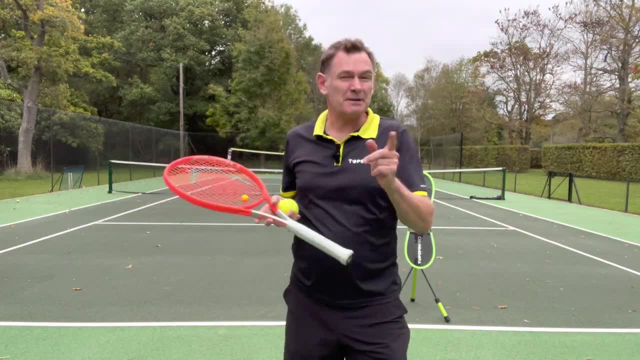 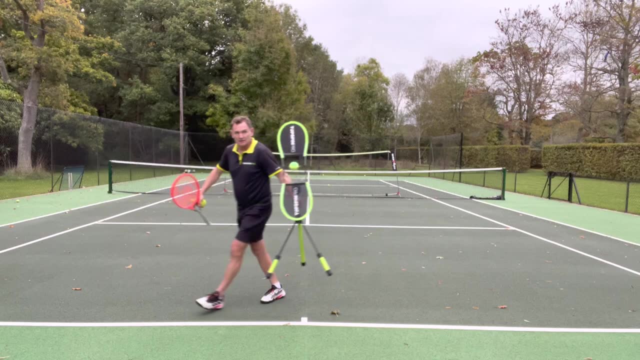 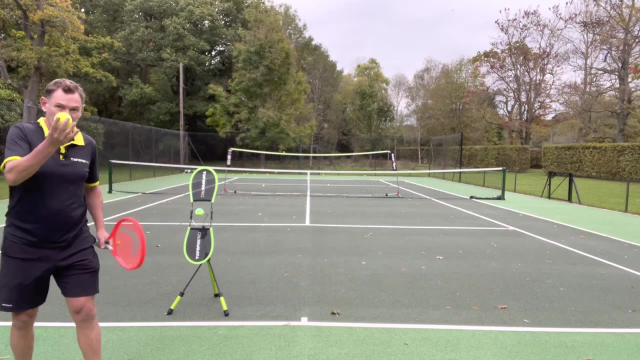 it going up and dipping down right at the back of the court. now the second part of this drill is to make it work for your backhand. so if you've got a single-handed backhand, uh, let's put Topspin Pro over there. um, it's a bit easier because you've got that spare hand to hold the ball. 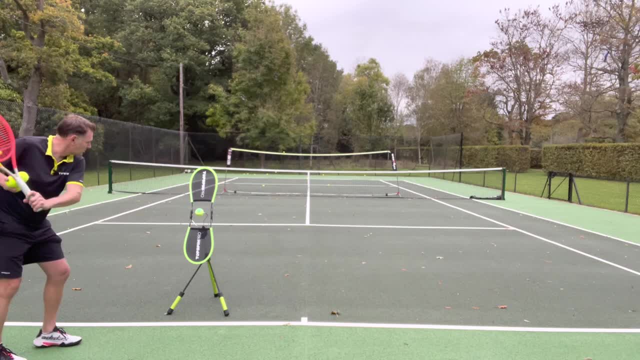 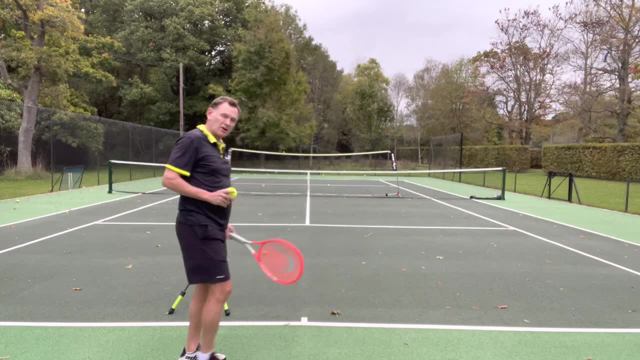 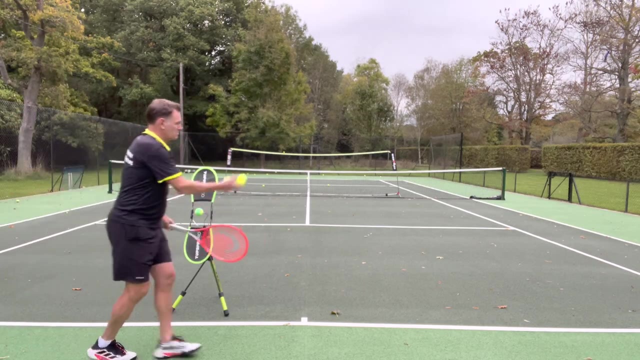 so same thing. you warm up the shot on the Topspin Pro and you run across, drop the ball and again got it over the first net and into the back box. so shot on the Topspin Pro, step across. that's a bit high right and that's fine. you want to practice. 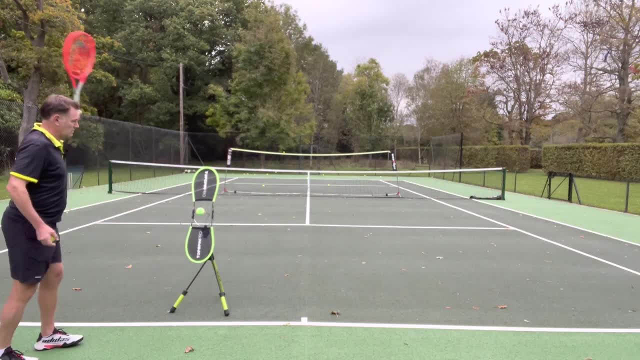 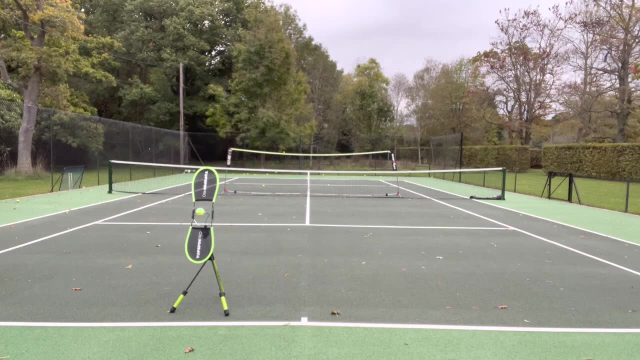 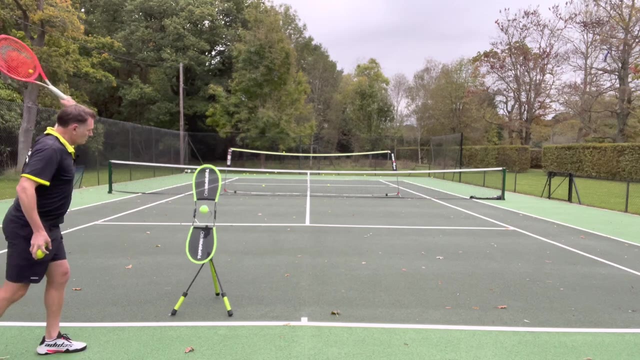 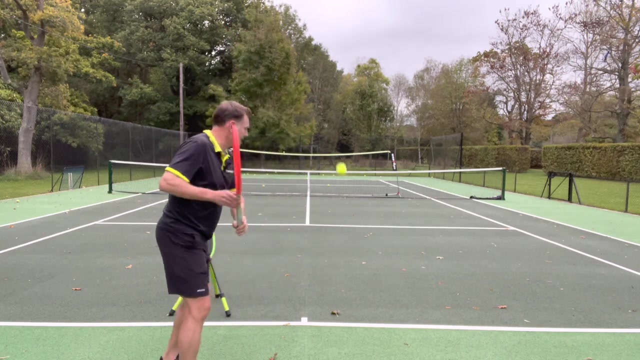 and you're going to get mistakes. so you keep going. Topspin Pro, step across again. that's long. I need more Topspin. let's see if I can do that right. so put more Topspin on the Topspin Pro. there you go, step across. yeah, much better. and one last one. 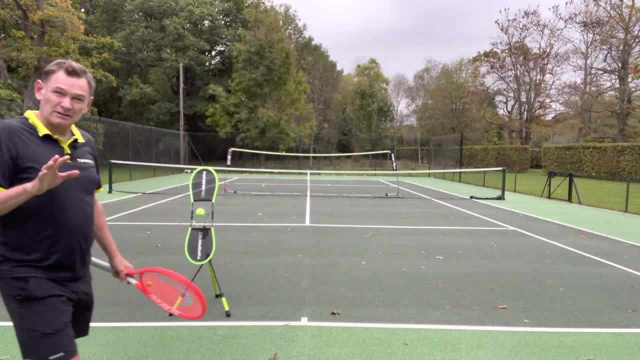 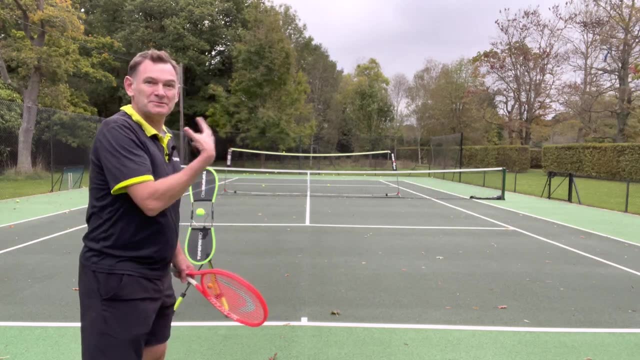 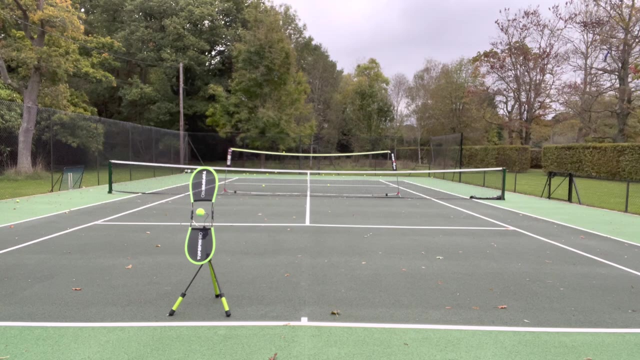 there we go, okay, and you can do it for the double handed backhand as well. it's a little bit hotter, so you've got to- uh, you've got to throw the ball with a bit more height, so you can- you've got time- get your grip and everything sorted out. let's try that now. so okay. so first the shot on the. 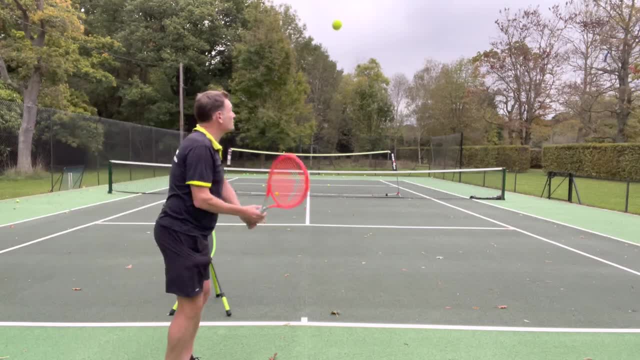 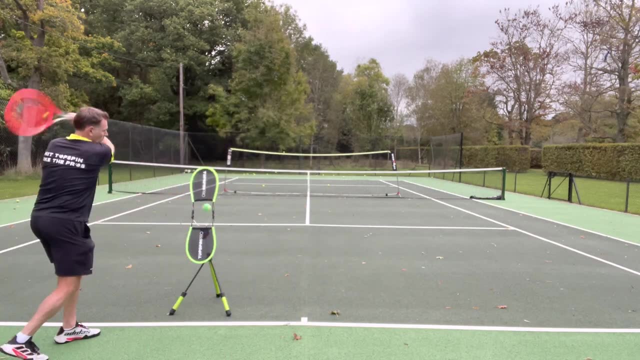 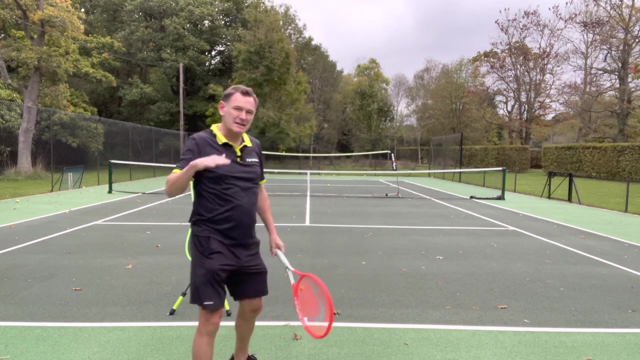 Tospin Pro. then you step across, toss it up. there we go. that one is a bit short. okay, again on the Tospin Pro, step across much better. and that shot, I mean that's deep, it's got a lot of Tospin, it's.